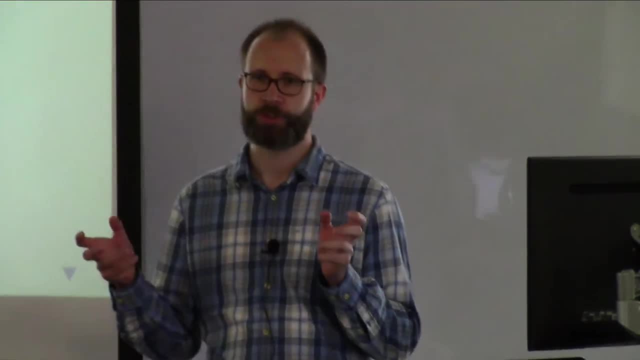 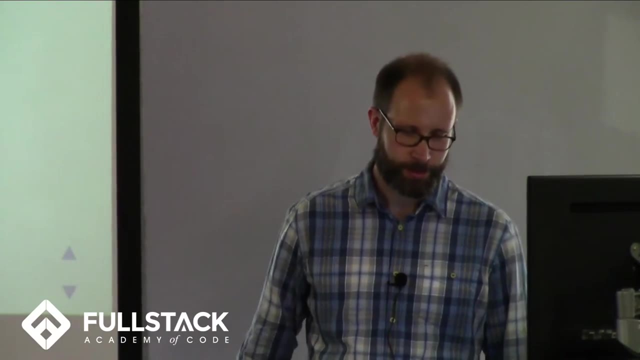 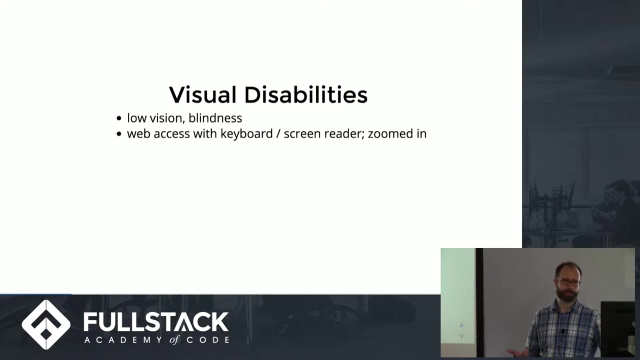 users with disabilities, which are visual disabilities and motor disabilities, and users with visual disabilities have low vision or are colorblind or are completely blind, and normally they access the internet with the keyboard in combination with the screen reader or, if they just don't see very well, they zoom in very much the web content. This is what they do. 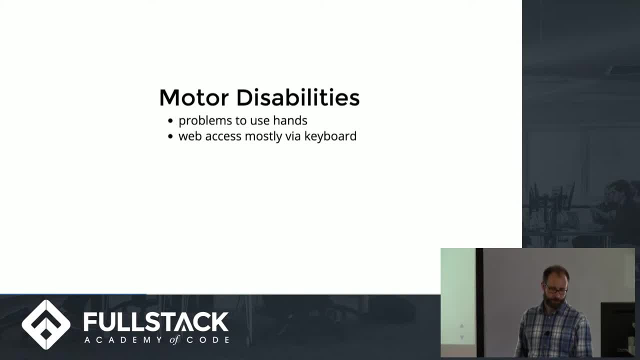 to get access to it. Users with motor disabilities normally cannot use their hands or have problems using their hands. for example, if they have a issue with their spine and they cannot, they can only use that they had moved their head. they cannot use the hands at all or they have just shaky. 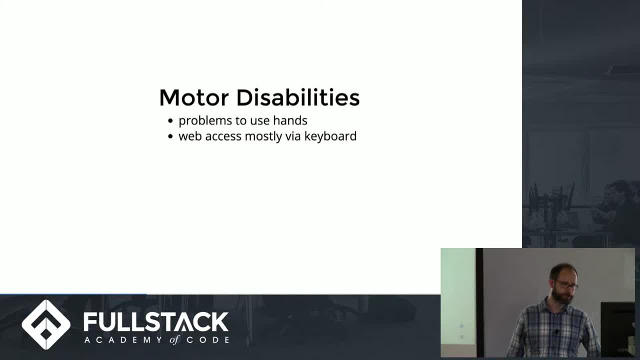 hands. so there's a problems for those users and they most of the time only use the keyboard to access the web. and here are some common problems that relate to these restricted access to the websites. so one is that people just want to zoom in to can better read the content, and 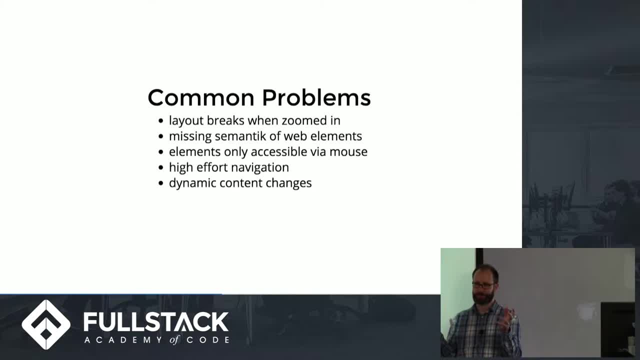 it can happen that the layout totally breaks when you do that on some web pages. that's one problem. Another problem is that the screen readers, the tools blind people use, only have access to the DOM elements so they can tell the user that they that there is an input. 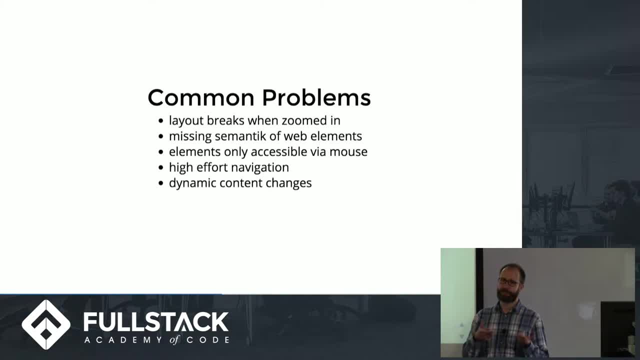 field or a button, but without a label or text for the button. they do not know what to put in the input field or what will happen when you click on the button, so there's meaning is missing for those elements. another problem is that you can have elements that are not accessible with the. 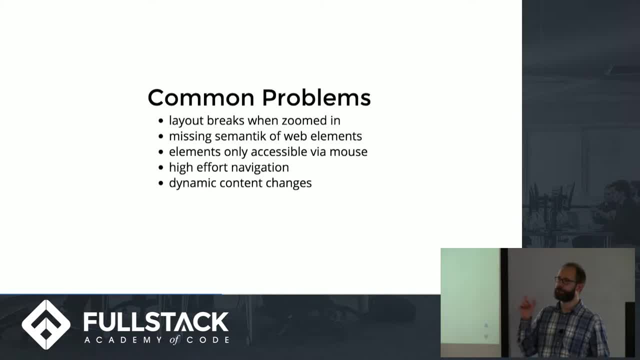 keyboard at all. so, for example, imagine you have a image element and you attach an event handler for clicks. you will not be able to reach that with the keyboard tap key, because normally only you can use can navigate to links or to form elements, but this image you will not reach high. 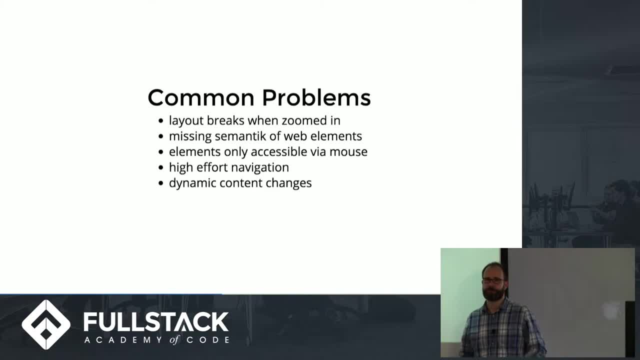 effort navigation. this is when you can imagine a normal website with a rich navigation on top and there is an input field in the main content area and the user can only use the keyboard once to reach that field and he starts. when you load the page, you start at the first element, which is normally link in the 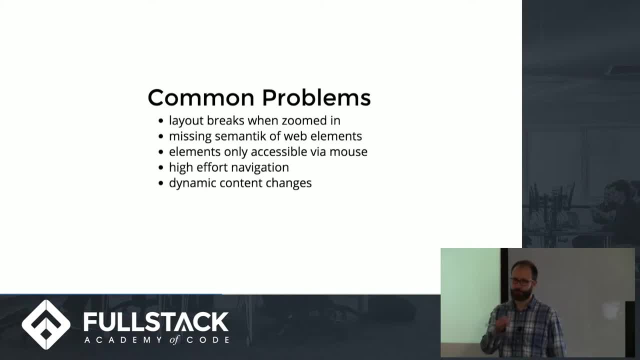 navigation. then you just click through the whole navigation links to reach that input field, which is a big effort for that user. and another problem is dynamic content changes. so all the websites we built in the last weeks are very dynamics. so, for example, you click a button here and over there the text of an 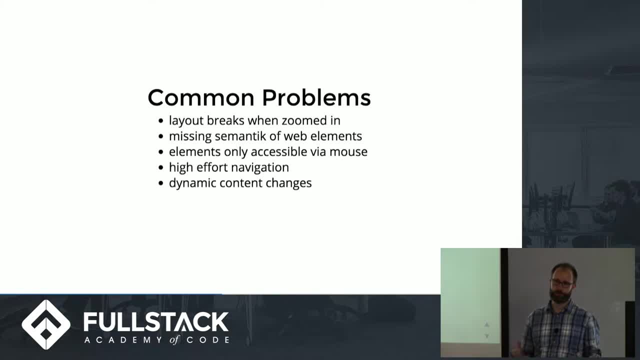 element changes and without doing anything, the screen reader will not recognize those changes and the blind user will not know what's going on here. so you have to do a lot of things. so this is just some examples I picked out which users with disabilities have to access web content. here are some solutions. one is called area- area stands. 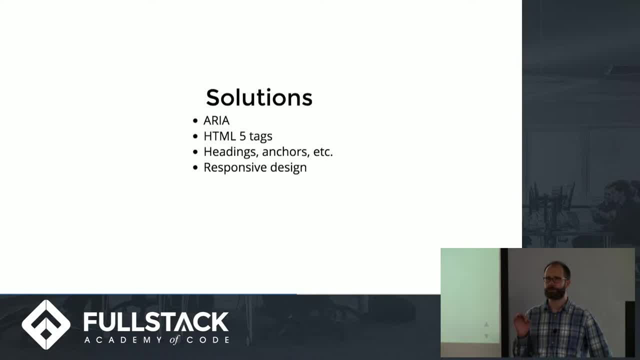 for access. accessible rich internet applications. yes, and this is just a specification which describes a way how you can make regular web elements more accessible in practice. in practice, this looks like it. it looks like that that you attach attributes to your elements. for example, you can have a input field. 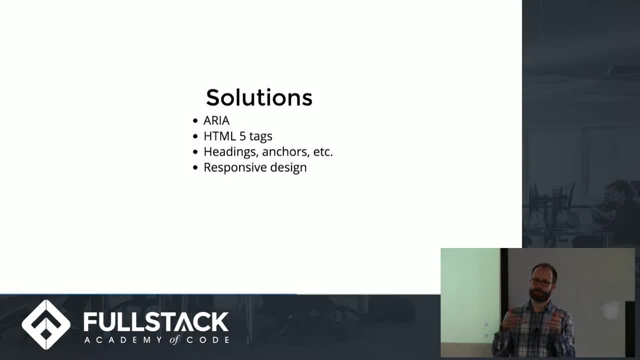 and just an attribute with a meaning, for that tells you what to fill in. or you have a button and you just had a label for it, so it tells the users what happens when you click on that button. and those attributes get picked up, so they will not change. 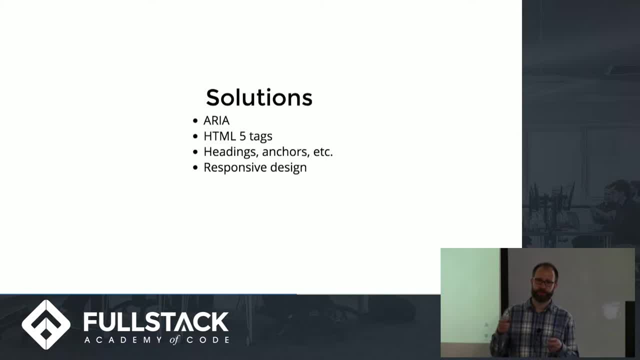 your, your the behavior of your website at all, but they get picked up from the screen reader and they will tell the user. they provide that information to the user. very similar HTML5 text like footer or main or nef, which is tell: okay, that element holds the navigation or that elements holds the footer, etc. you 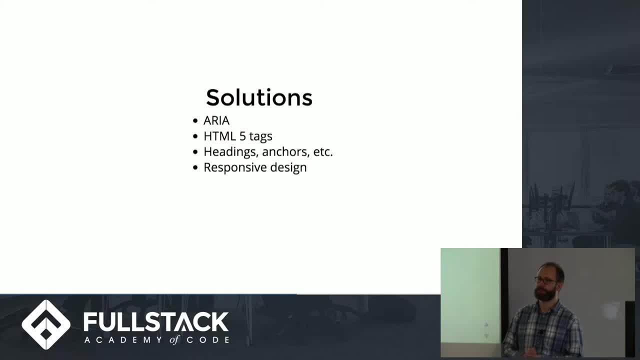 can use headings to structure your website and this also enables users with using screen readers to better navigate through the page. you can use anchors to create shortcuts, people using the keyboard and so on, and, of course, you can use responsive design for people who want to you zoom that they. 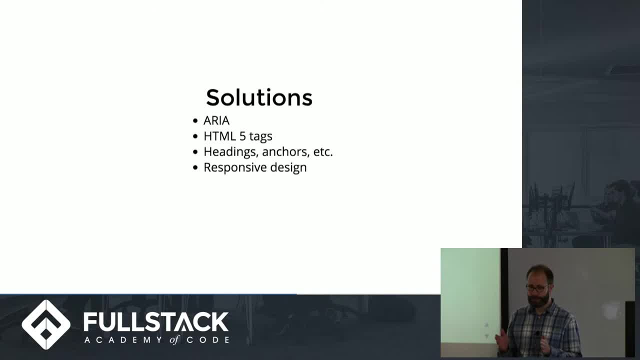 have a still a nice layout which is not broken, and I figured out that. alright, I found something that you can disable this zooming functionality at all, and I think that's not a good thing and you might want to check the others for that. and I think there's a few things there, but nothing great there for testing all and this they're. 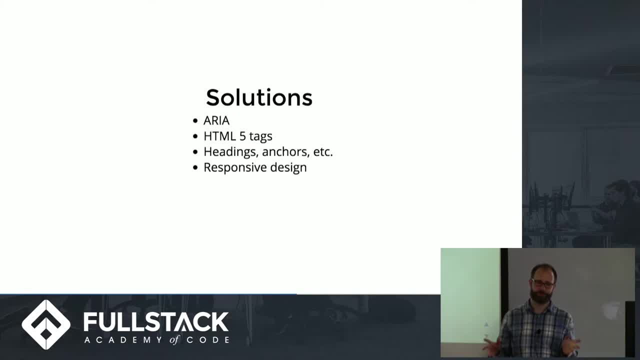 you shouldn't use that. You can say, OK, I have implemented everything And I know that the user is using a desktop monitor And it should look good on a desktop monitor, But still people may not be able to read it. 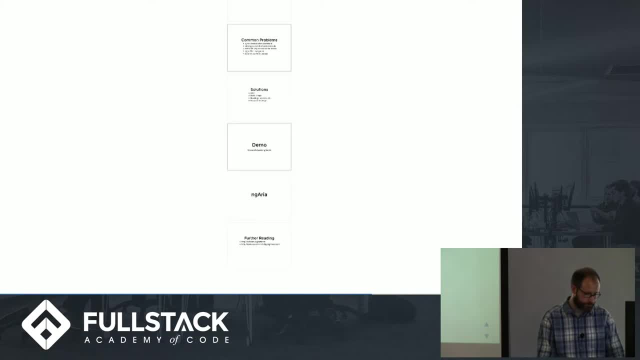 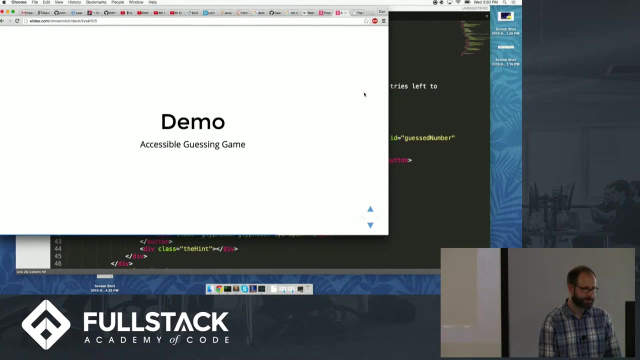 OK, I've prepared a little demo that shows you an application. How do I leave the Command-Shift-F? Command-Shift-F? OK, thank you, So I will show you. So this is the guessing game I wrote during Foundations. 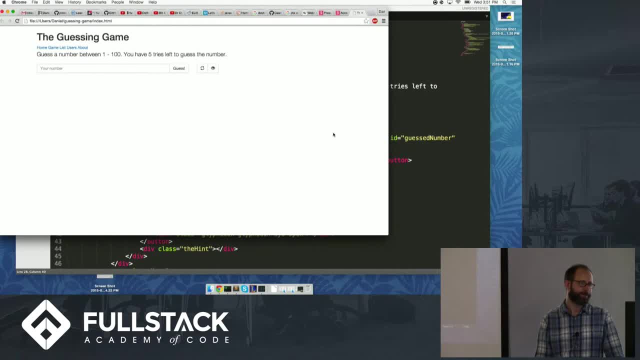 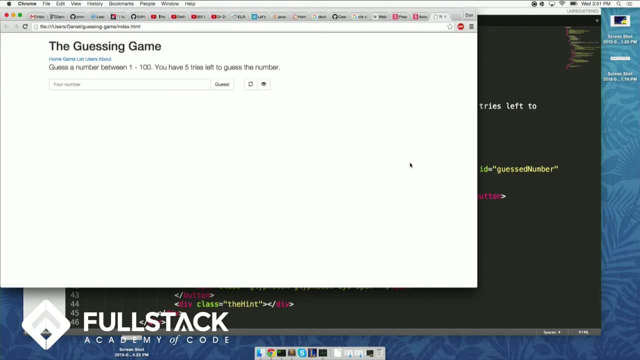 And it has some accessibility issues And we are trying now to fix them. So what I will do is I will fire up a voiceover, which is the screen reader that comes with the Mac, And I want you to carefully listen what it's reading out. 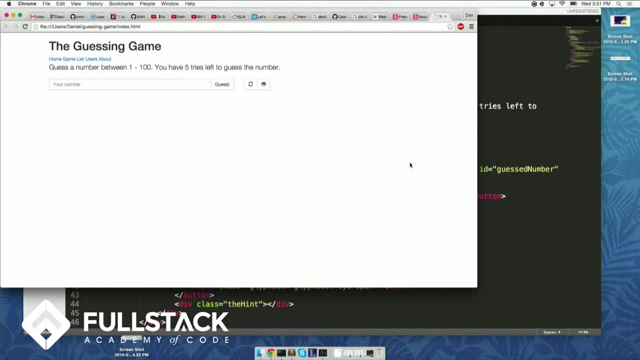 especially when I'm over the input field and when I'm over the buttons. Voice over on The guessing game is handed to number one Link gameless. So here I can control where it should go. Link link Guess a number between 1, 1, 0, 0. 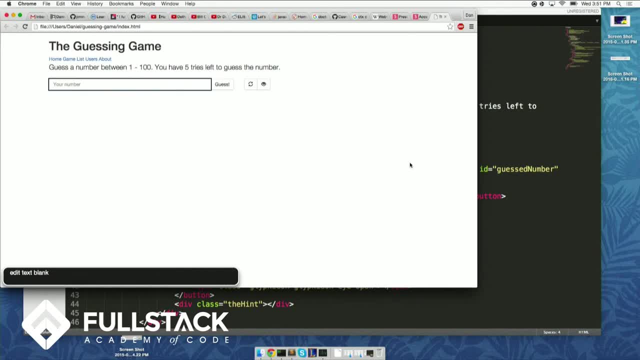 You have five tries left. You have to guess the number. Edit text: Black Guess Black, Black, Black, Black. So you can see I'll turn it off. I'll turn it off because let's keep on speaking. 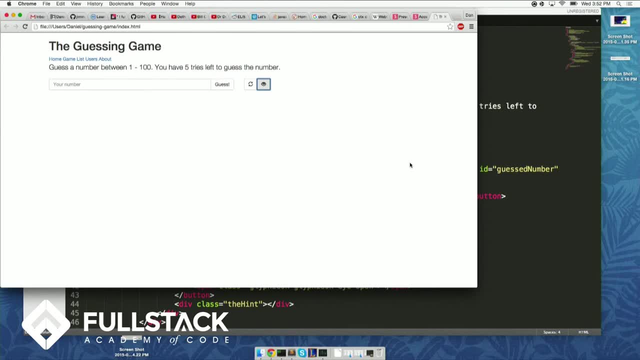 You can see it just says button, button and input field edit text. So there's absolutely no meaning attached to it for the user. The user doesn't know what it means when it clicks on the button, et cetera. OK. 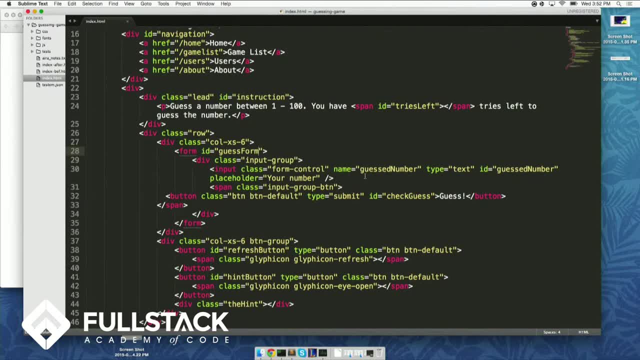 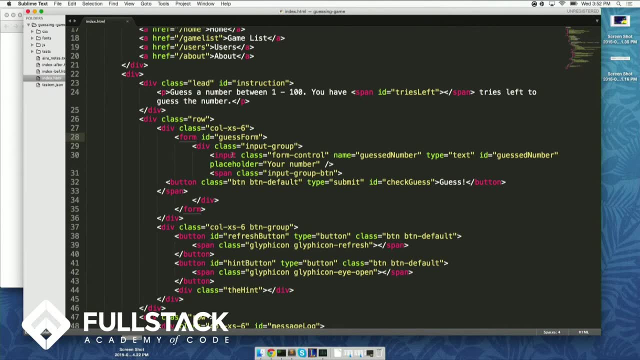 But it's very easy to fix that. As I mentioned before, you can use area text to put a meaning on those fields, And here I'm on the input field and I'm going to just use something like called area label. Let me see. 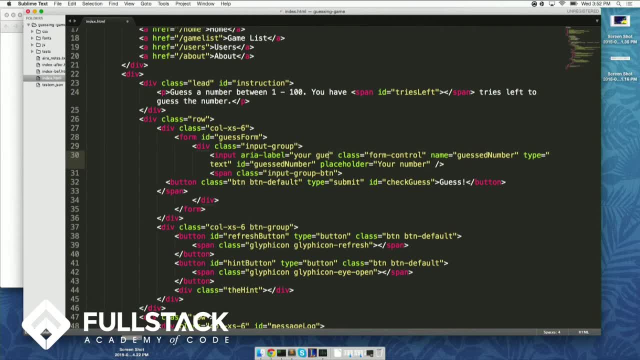 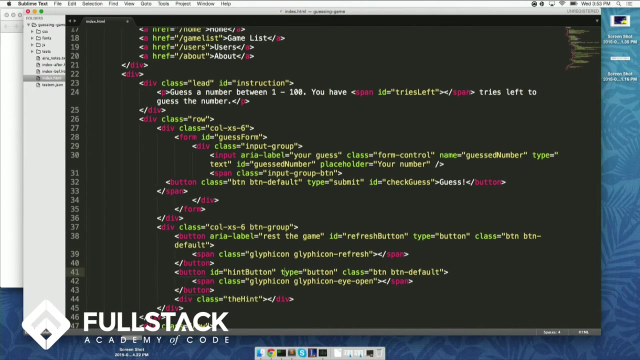 Oh, it's there Like your guess. OK, And I will add the same at the button with a different value. So here's that button. Just what is it doing? Reset the game And the other one. It's just show the hint. 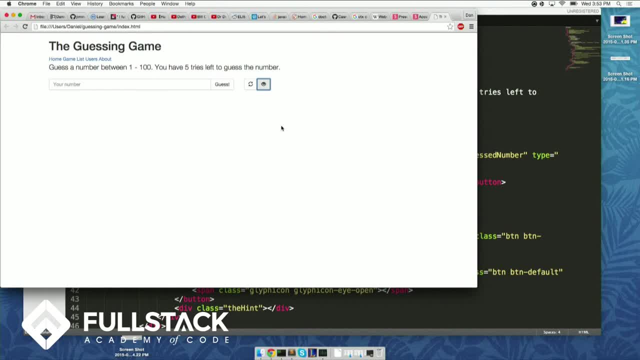 OK, Save it. I'll fire it up again and navigate over those input fields and buttons to see what it's reading. Voice of the guessing game: Your guess. edit text: Guess: OK, Rest the game. OK, Little typo. 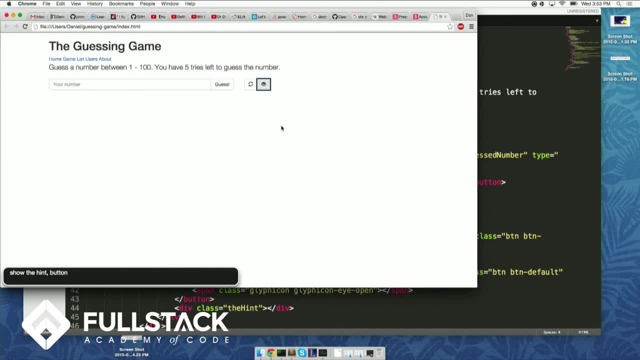 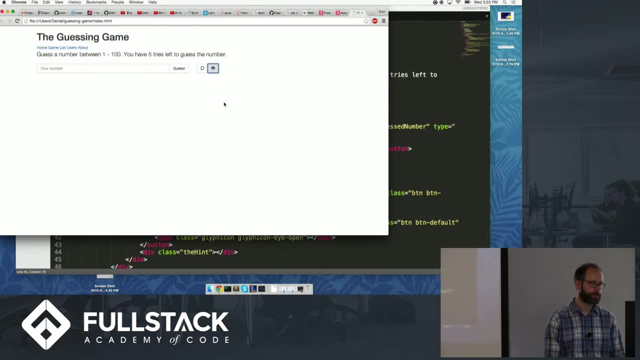 Sure, But you can guess. But you can guess, You figure out how it works, right, OK, And not. So now the user knows. OK, Here I put in the number And there is the button to make the guess. 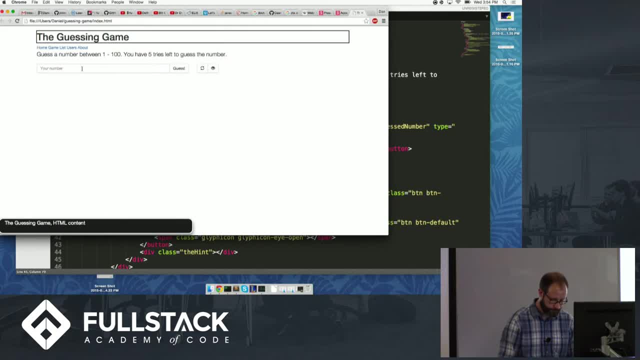 And if you do it now, Voice of the guessing game: Html Link. Link Your guess. Edit text: 3, 4, 3, 34.. OK, So you can see. So you can see. in this state the game has no purpose for that user because he's putting. 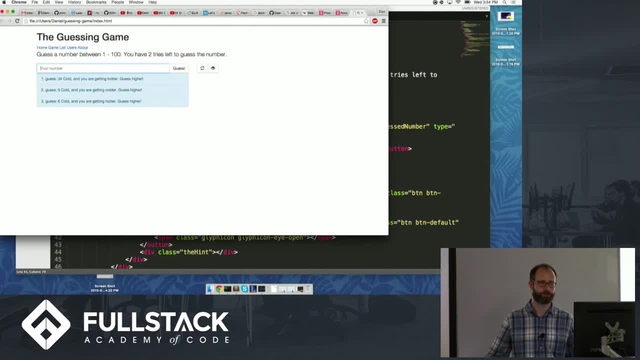 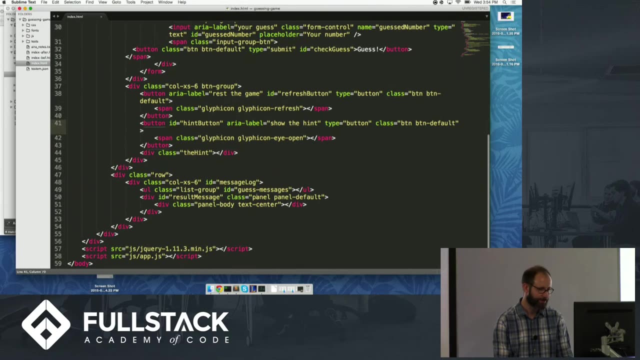 in the numbers, But he has no idea what's happening, right, Because One second, OK, You can wrap up, Yeah, So it's very easy to fix that. I think it's very important to make that one thing, And afterwards I will not take any questions.